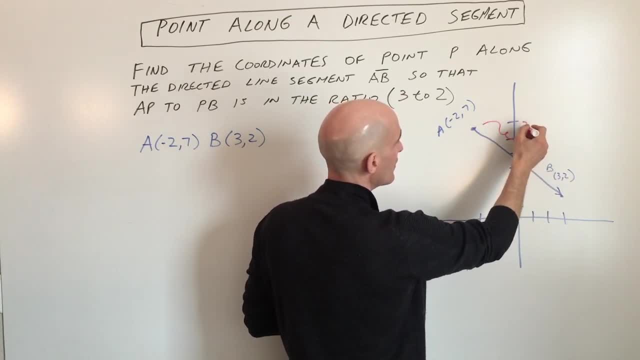 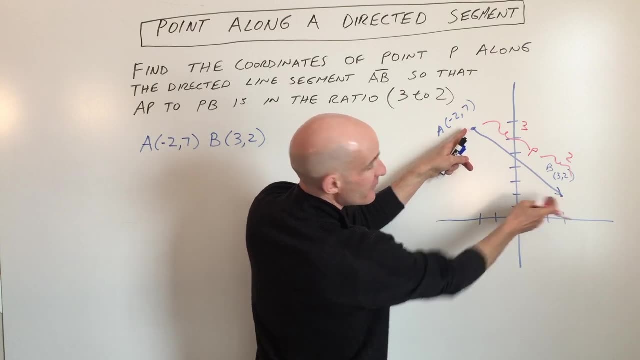 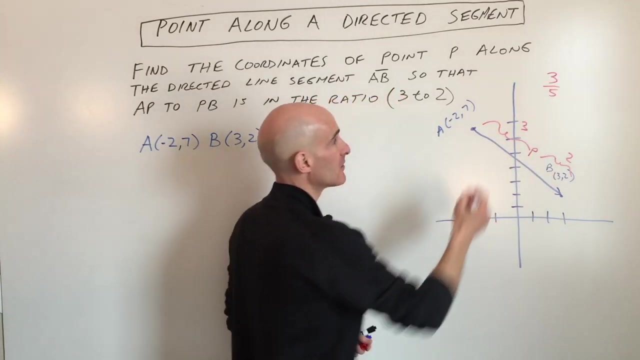 don't know, somewhere along this line, but we want that ratio here to be 3 to 2.. So what that means is you're heading 3 fifths of the distance from A to P, So I'm just going to write that 3 fifths of the way. okay, So I added these together 3 parts out of 5.. So 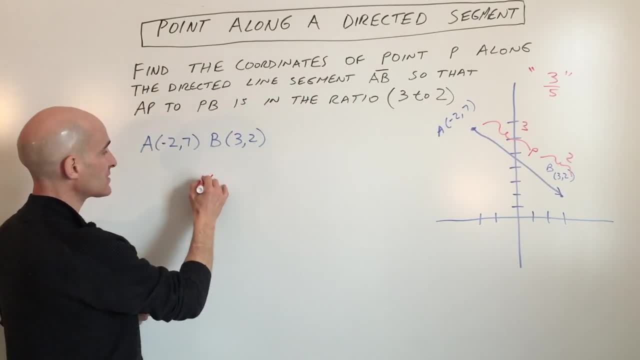 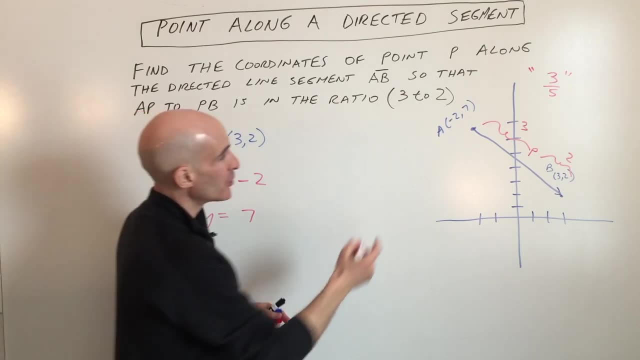 what I'm going to do here is I'm going to say, okay, for X, the X coordinate of point P, we're starting out at negative 2.. For the Y coordinate, we're starting out at 7.. But look what's happening, We're going to be going down. so 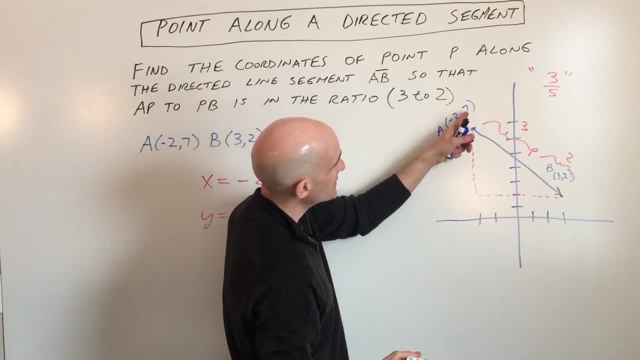 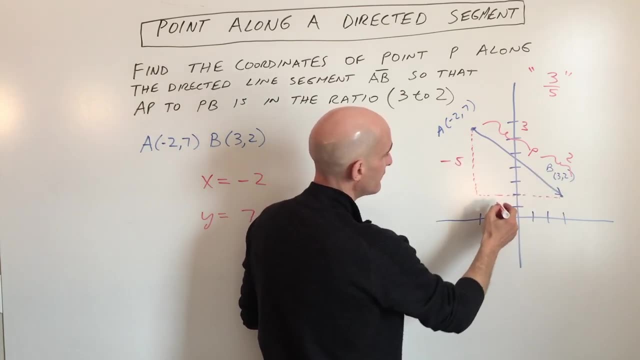 much over so much. So we're going down 7 minus 2, which is 5.. So we're going down 5, okay, And we're going right 5, okay. So down 5 and right 5.. So this is going to affect. 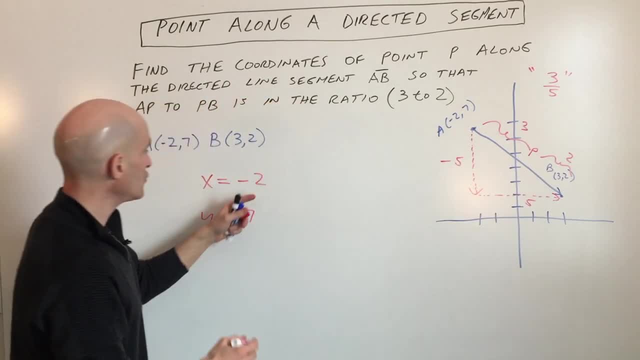 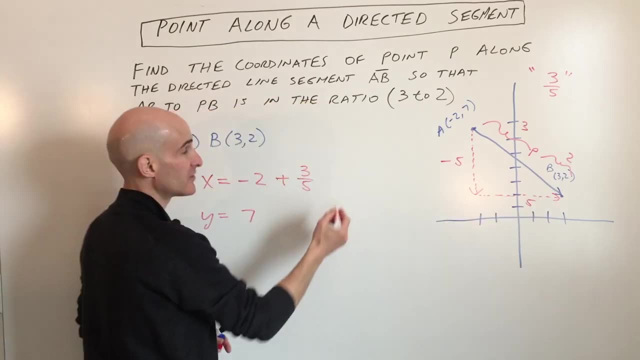 the Y coordinate. This is going to affect the X coordinate. So what I'm going to do now is I'm going to to the X coordinate, I'm going to add 5.. 3 fifths, remember 3 fifths of this horizontal distance. So 3 fifths of 5, okay, And for 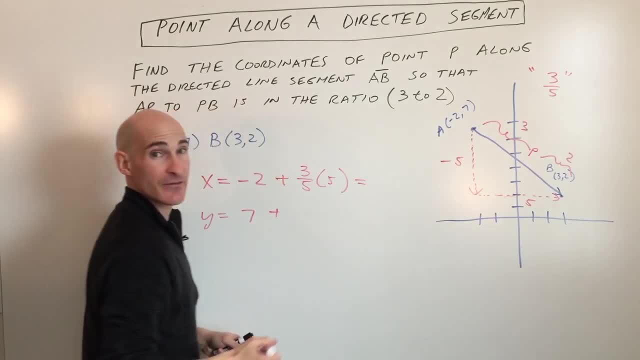 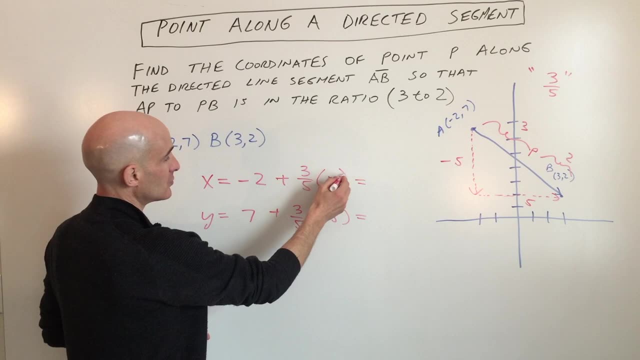 the Y, I'm going to add 3 fifths of negative 5, since we're going down 5.. So 3 parts out of 5 out of negative 5.. So this is going to come out to 3 minus 2, which is 1.. These are